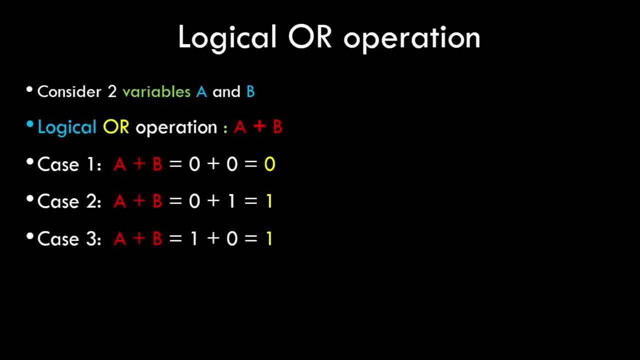 let's see case 3.. Let's try consider example 4, where we consider a is value to be 1, and b is value to be 0. Again, 1 or 0 is equal to 1.. Let see case 4, where we consider a and b are both to be. 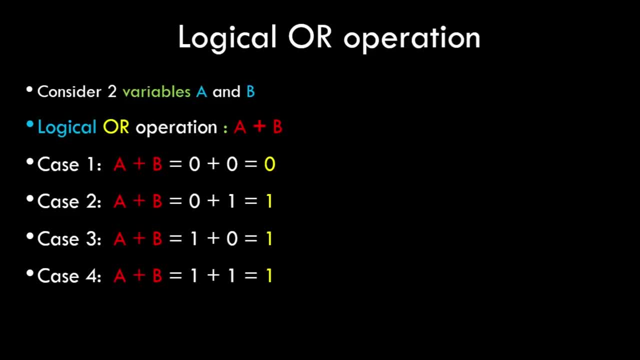 1.. So now we have 1 or 1 is equal to 1.. Now this is different from the typical algebraic addition operation where we have 1 plus 1 equal to 2, but the logical OR operation between 1 or 1 give us again 1.. Now, to summarize all these cases, We have a logical OR operation which gives us 1ーブ1.. To summarize all these cases, we have a logical OR operation which gives us again 1ーブ1.. If we analyze all these cases, we have a logical OR operation between 1 or 1 is equal to 1.. which? 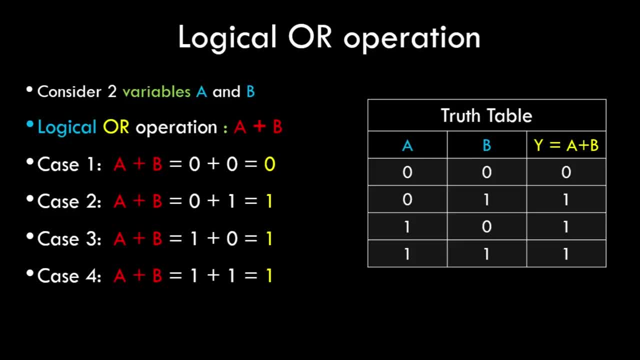 have a truth table. A truth table is a table which has all the possible inputs of the variables and its corresponding outputs. So, as you can see, the first two columns are the variables a and b, with the different values, and the third column y, which is the output or the 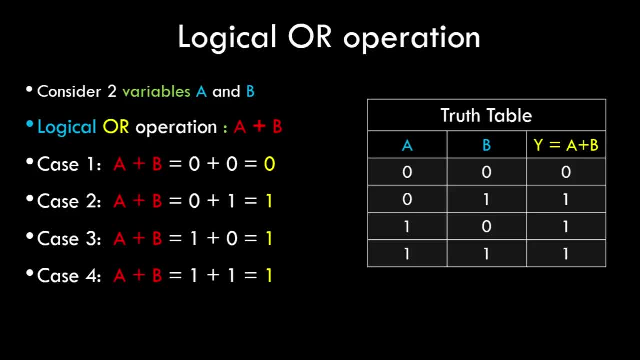 right hand side, which is the operation a or b. So we will be using these truth table values and we will be drawing these truth tables in our further tutorials as well, when we solve some numericals. Ok, so now let's have a look at logical and operation. We again consider: 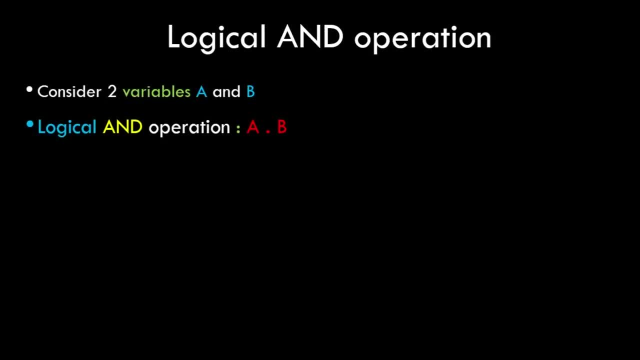 two variables, a and b. Now the logical and operation is denoted by the symbol dot between the two variables and it is pronounced as a and b. So again we will have these four cases. For the case 1, we have a and b value to be 0. Now this logical and operation works. 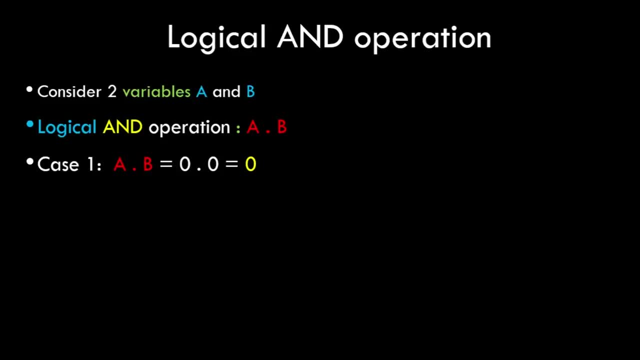 like a algebraic multiplication. So 0 and 0 will give us 0.. Consider case 2, we will consider b's value to be 1.. So 0 and 1 is again equal to 0, because if we consider it. 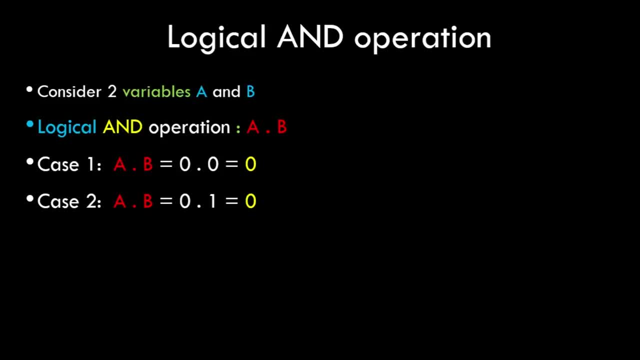 to be a similar, as multiplication value 1 into 0 will always give us 0.. Let's see case 3, we consider a's value to be 1 and b's value to be 0. So 1 and 0 will give us 0 again. 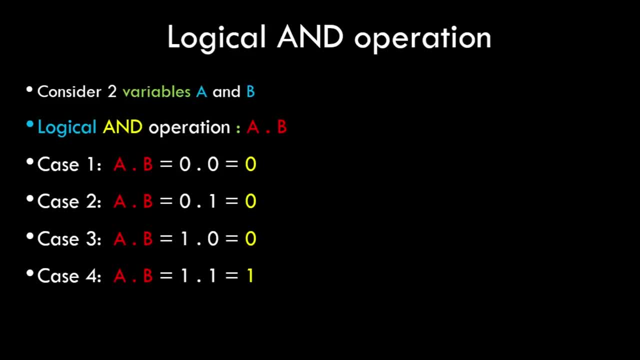 In the last case, where we consider both a and b to be 1, the value or the answer 1.. Since 1 and 1 is equal to 1.. Now summarising all these cases in the form of truth table, so we have the first and second column to be 1 and the answer to be 1 is 1.. Now in the